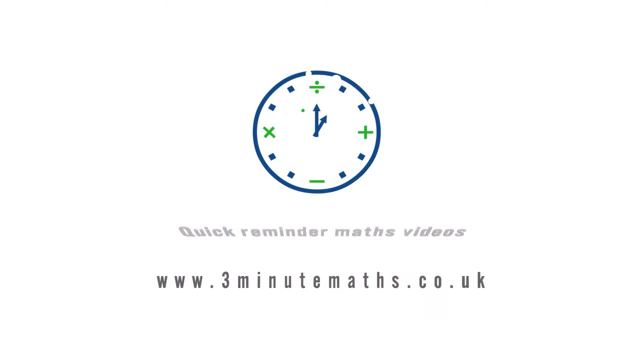 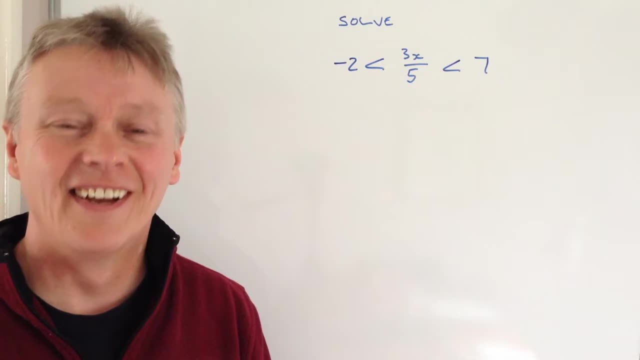 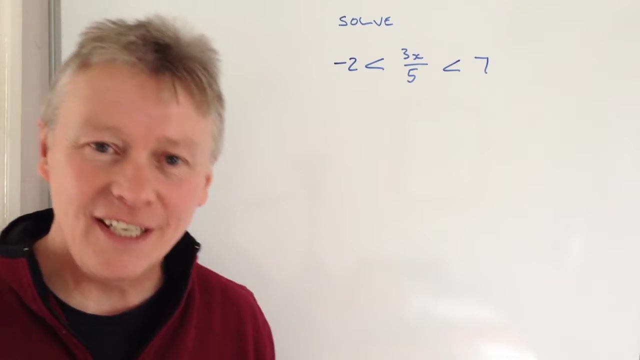 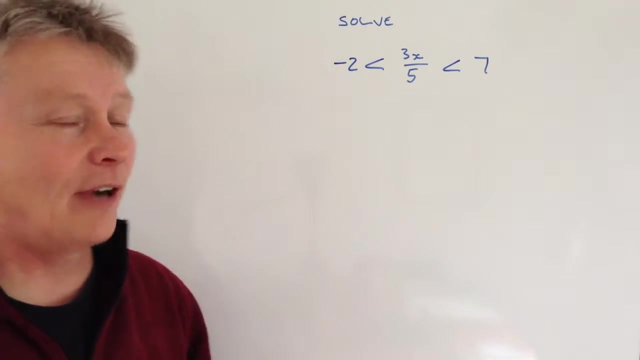 Hi, this particular video is towards the end of the playlist on solving inequalities. It's going to be round about an A grade GCSE at probably round about level 7 on the new curriculum. What it's asking us to do is to solve for x, in other words, find the value that's bounded. 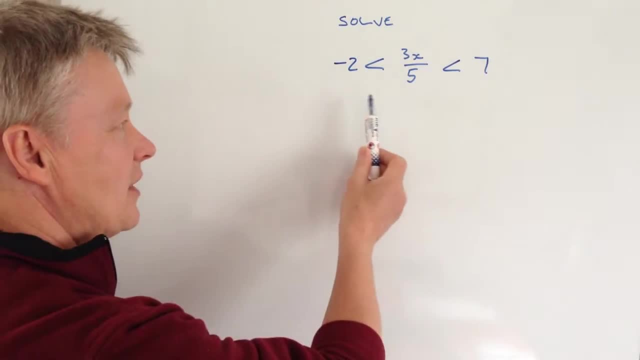 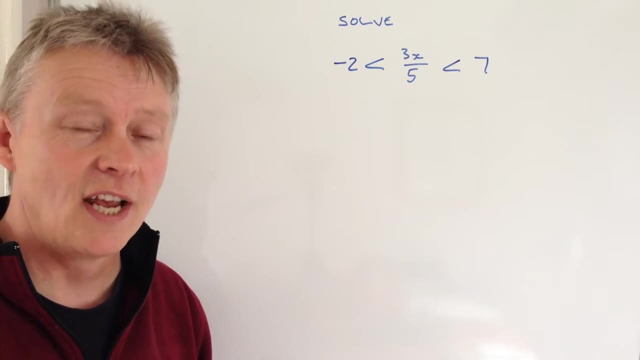 by this particular inequality. So the way to do that is that I'm going to treat the two sides as completely separate and then I'm going to treat them both as linear equations. If you're not sure about how to do that, have a look at the playlist on linear equations. 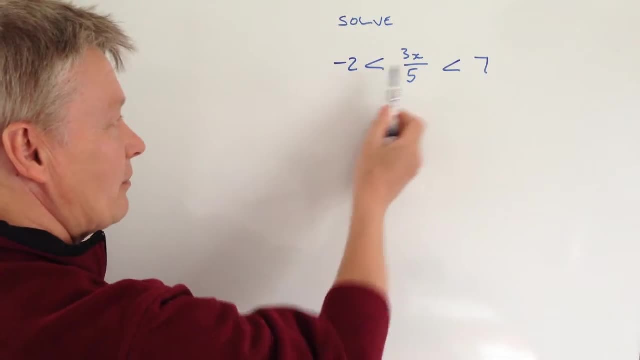 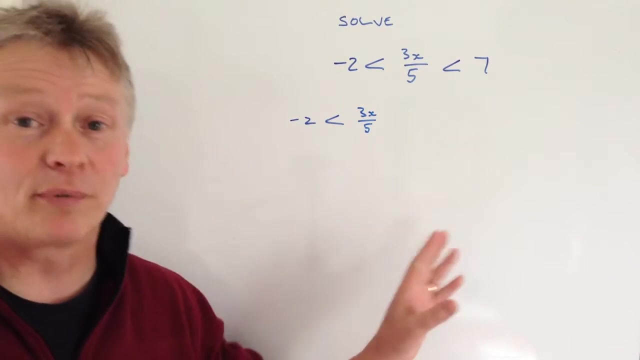 and you'll be able to hopefully follow this through. But what I'm going to do is I'm going to say minus 2 is less than 3x over 5 and at this point I'm going to completely ignore the right hand side of the inequality. 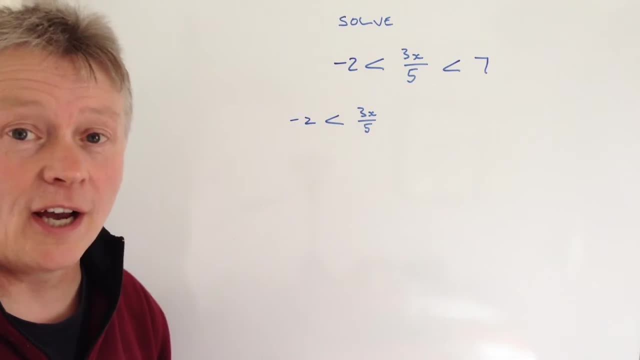 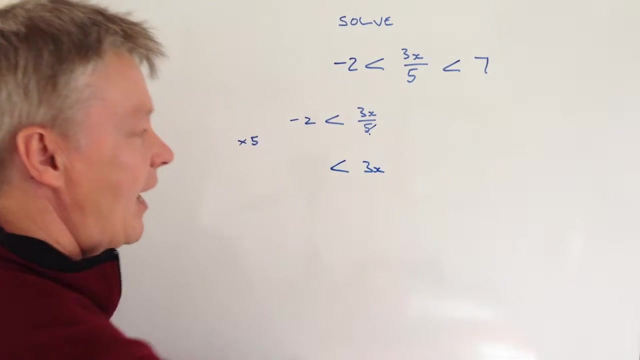 So on this side I've got a denominator of 5.. Well, it's just kind of easier if I get rid of that denominator. So I'm going to multiply both sides through by 5, because if I do that it means I can lose that one and I just get on the right hand side 3x On the left hand. 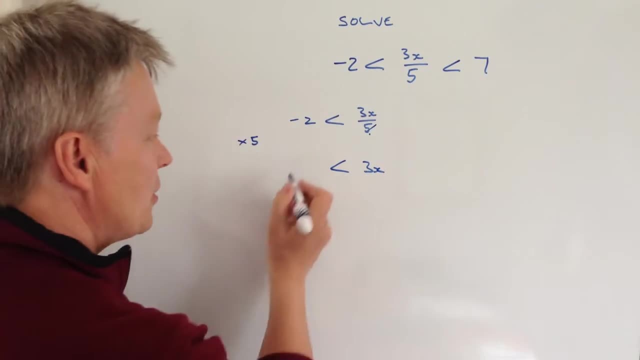 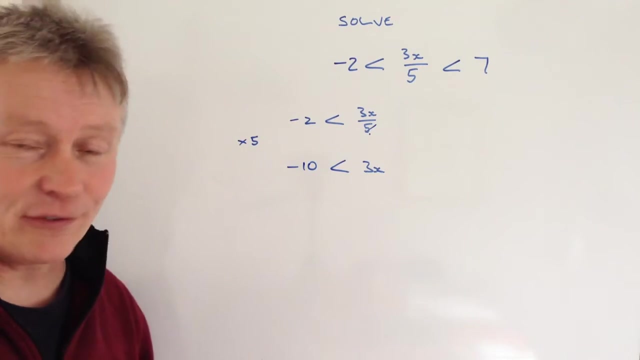 side, I get times 5, times minus 2, which is going to be minus 10.. Okay, so I've got minus. 10 is less than 3x, 3x. Okay so now I've got the two values of x, so I need to get one value of x. So what I'm? 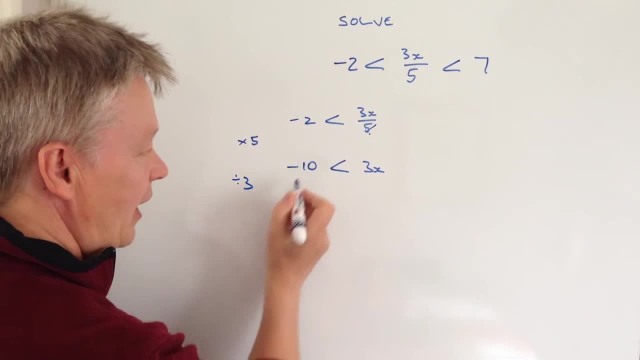 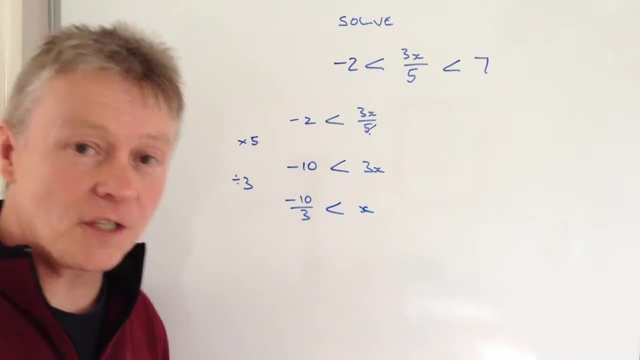 going to do is divide both sides through by 3.. If I do that, on the left hand side, I get minus 10 over 3, and on the right hand side, I just get x on its own, which is exactly right for what I'm looking for- Excellent. So now what I need to do is do exactly the 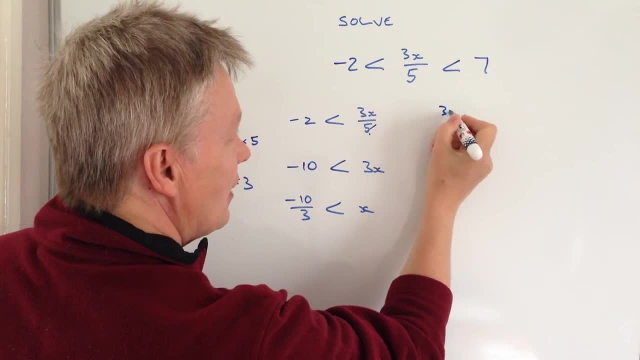 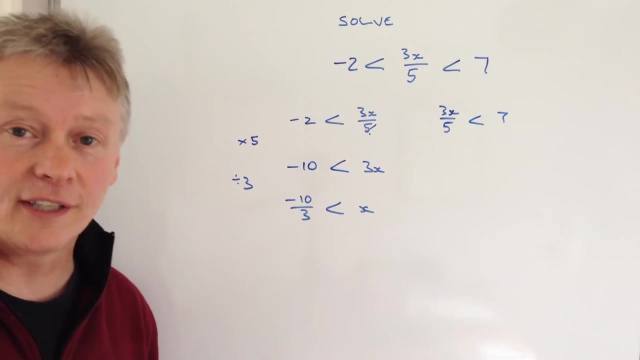 same on the right hand side. So I can write that as 3x over 5 and that's less than 7.. Well, again it, in the same way as a linear equation. I'm going to multiply both sides through by 5, because if I 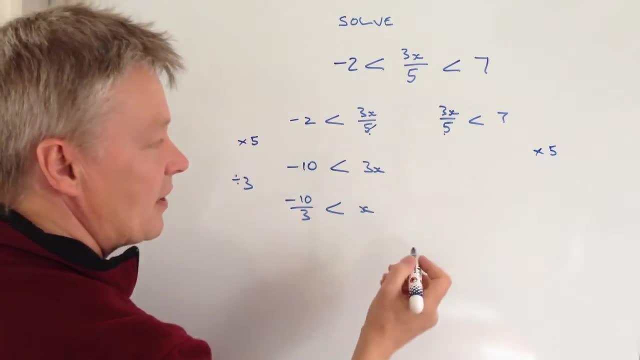 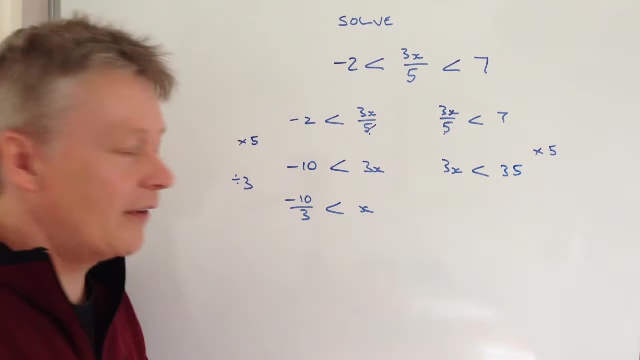 do that, I get rid of this denominator and on the left hand side then I get: 3x is less than 7 times 5 is 35. so I've got three lots of x is 35. I want to get one lot of x, so I'm just again going to.